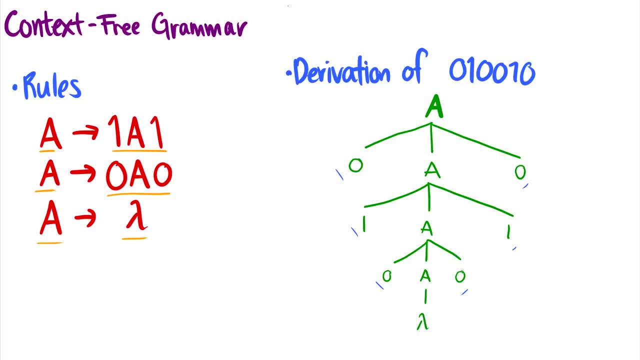 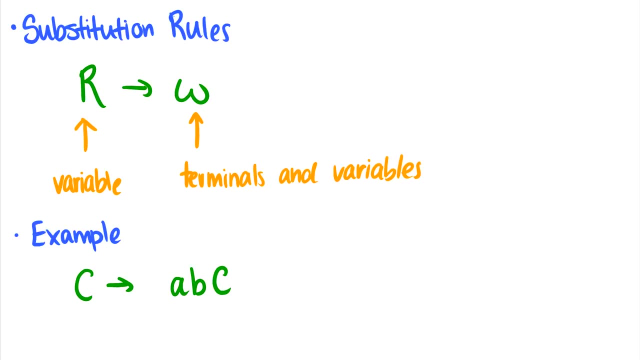 0, 1 0, 0, 1 0.. So context-free grammars allow us to do these palindromes, which is really cool, and we can see it's much more powerful than regular expressions already. So the rules are called substitution rules and essentially it takes a variable, which we'll call r for this case, and it 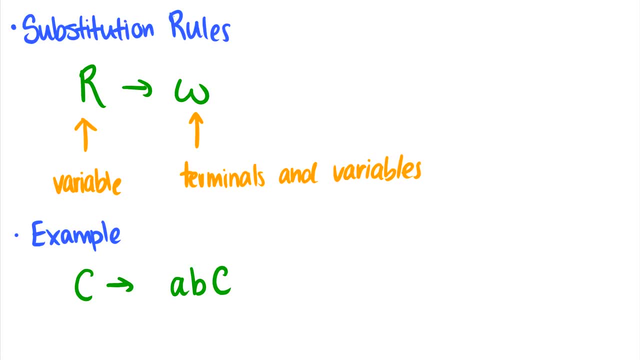 sends it to or rewrites it, substitutes it with terminals and variables, so some string w. So it is written that the variable here r is always a variable or a non-terminal. and on the right it doesn't matter what we have, So we can have a going to a b where it just goes from the variable a. 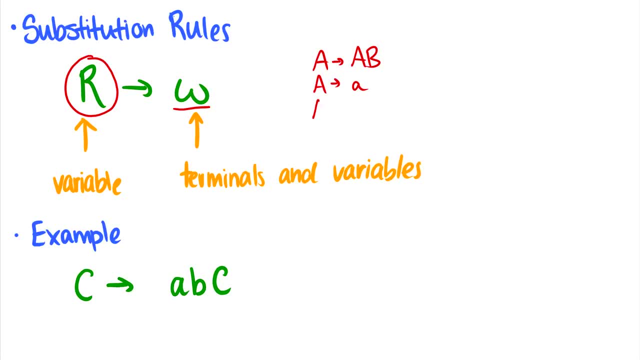 We could have a going to some terminal a or we could have a going to a combination of both. So another example down here is the variable c going to terminals a, b and another variable c. So if I were to draw this in a tree it would look like this: So a- b. 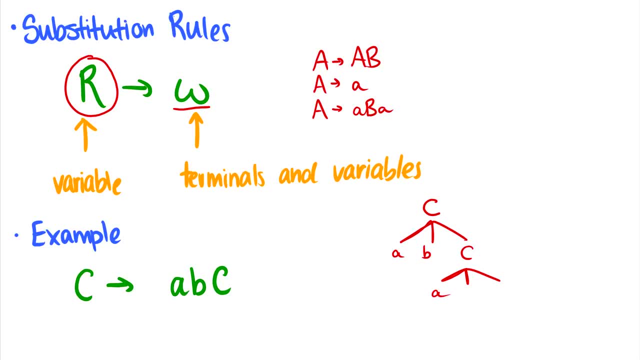 then another terminal c, and then we could repeat recursively and indefinitely, since there's no way to terminate this tree since, as we can see, c is in the input and the output. this will never terminate, which means we also have to have another rule that c goes to lambda at some point, in order. 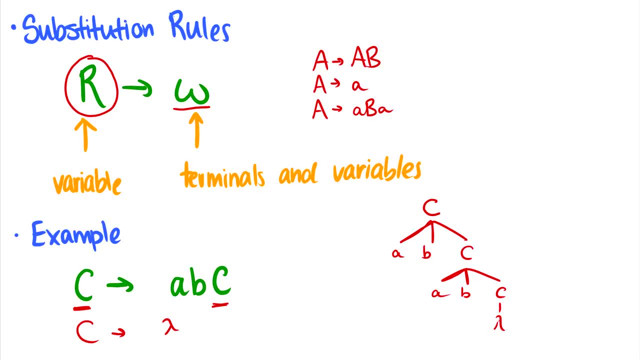 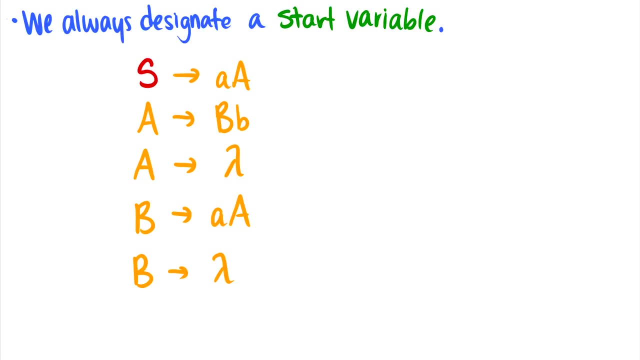 to terminate it, But you can see with this rule that we get pairs a, b star. Okay, there's a couple important things with context-free grammars. The first important thing is that we always have to designate a start variable. So that is what. 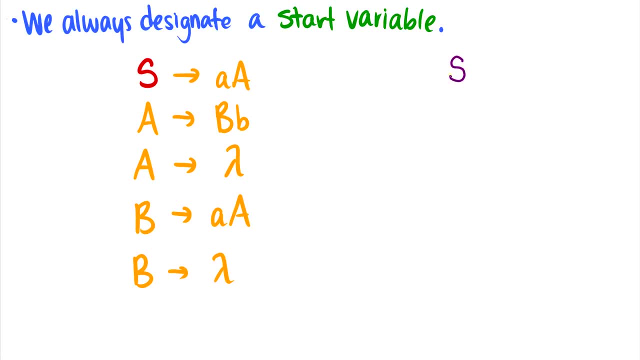 we start the derivation with. In this case it's s, and usually I will use s for a start variable, but we could start it with anything we want. The important part here to note that with a start variable is that the start variable will usually just start the derivation with a start variable. 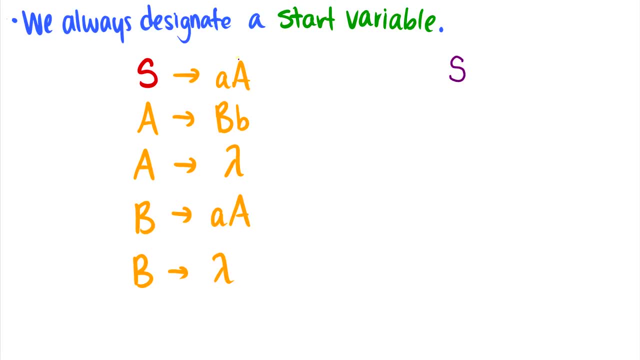 So it won't send itself to other variables. it won't normally send it back to itself, and this is usually a nice way to avoid having infinite regressions where you can never terminate your tree. but it's not necessary. So it is possible to have another rule that goes s to a s and then. 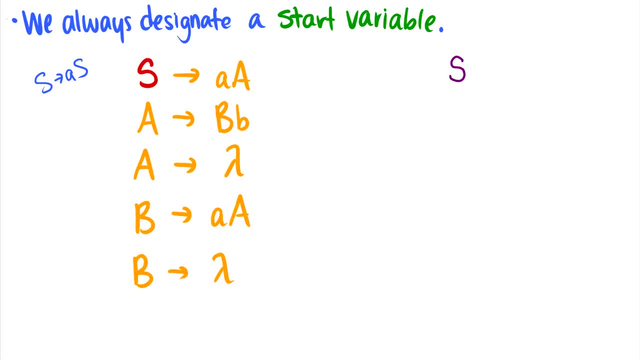 s to a a, and then we could recursively go on s as much as we want, but sometimes it's a good idea just to have s starting the derivation and then sending it to another rule, just so we explicitly know what the start variable is. For the most part, we won't ever state it. we'll just assume that s is. 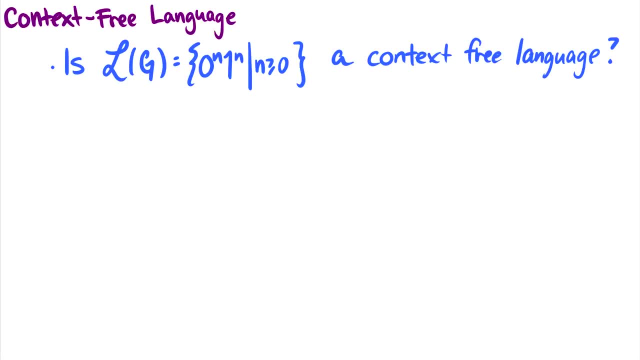 the start variable. So here's a question: Is the language of g equal to 0 to the n, 1 to the n, where n is greater or equal to 0, a context-free language? Now we have shown in regular expressions that this is not possible using the pumping lemma, but can we do it with a context-free language? And the answer: 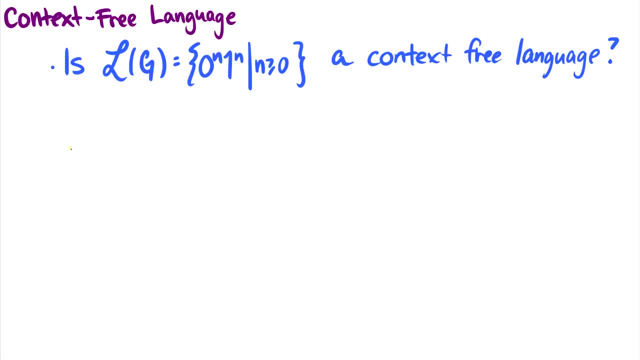 is yes. So there's really just one rule we need here, and that is that a, which we'll call a, as our start variable. but we can have a rule that goes from s to a to start ourselves off. We'll have a go to 0, a, 1 and then 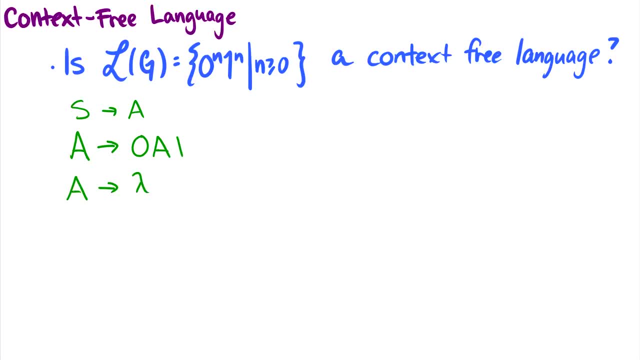 we'll have a terminating symbol. a goes to lambda. Now let's see how this works. Let's do the case where n is equal to 0. So we have s, s goes to a, and then a goes to lambda, and now we have a 0 to the 0,, 1 to the 0.. Let's do 0 to the 1,, 1 to the 1.. We can have s going to a to start off. 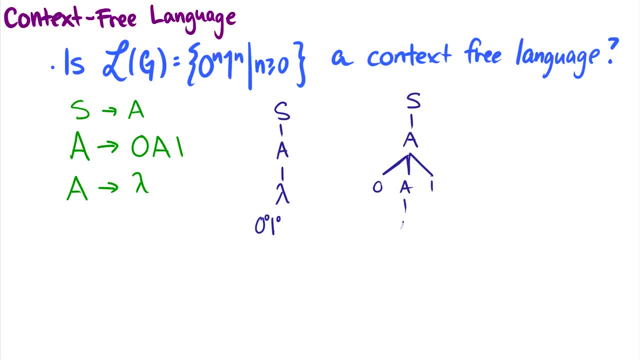 then we'll go 0 a 1 and then we'll terminate it with lambda. So that is 0 to the 1,, 1 to the 1.. But we can keep going. We can just take this a and keep splitting it into ternary branches: 0 a 1,. 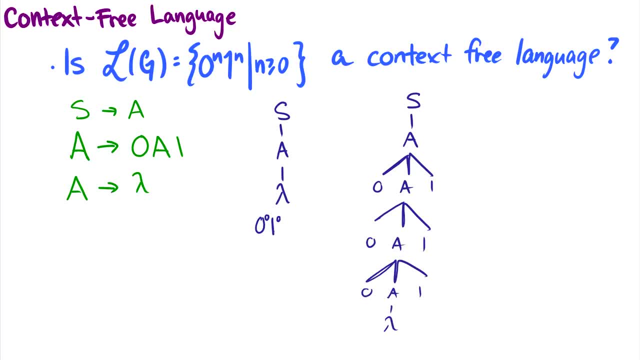 0, a 1 and then stop. So now this is 0 to the 3,, 1 to the 3.. So with context-free language, we can generate these languages, such as 0 to the n, 1 to the n. So it is a context-free language. 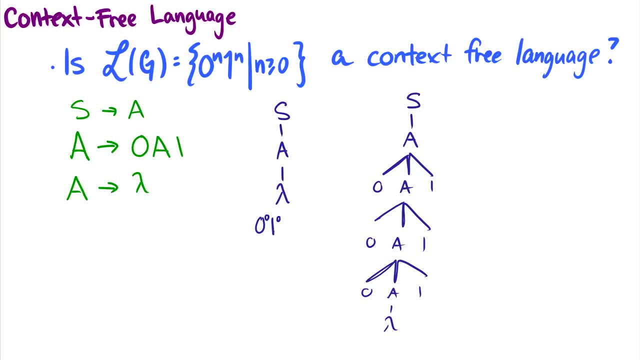 And this is the power that context-free languages give us, So we can fix some of the problems in the human language is not regular video using context-free languages. So, for instance, we can have the center embedding across serial dependencies with this, where we have n nps followed by n vps. 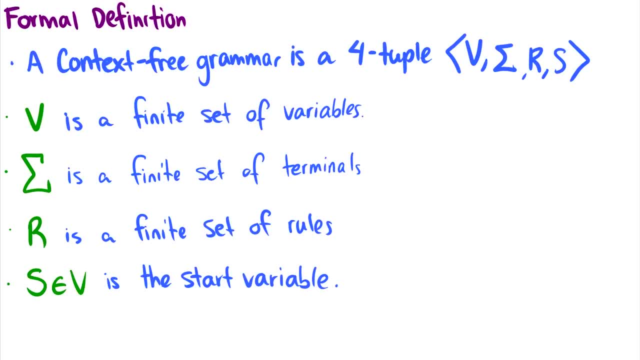 Okay, now I'll jump into a formal definition of a context-free grammar. So a context-free grammar is a four tuple v, sigma rs, where v is a finite set of variables. We denote these with capital letters, usually a, b, c and so on. Typically in rules I will use r as a default. 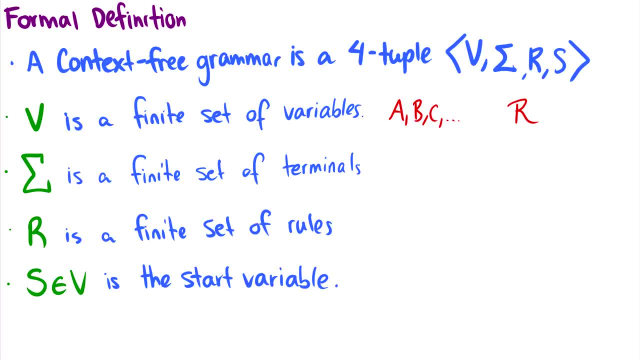 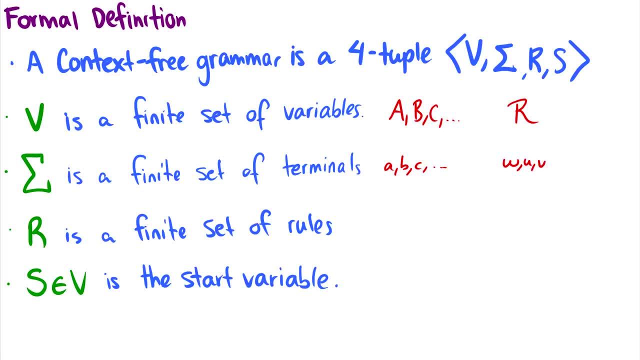 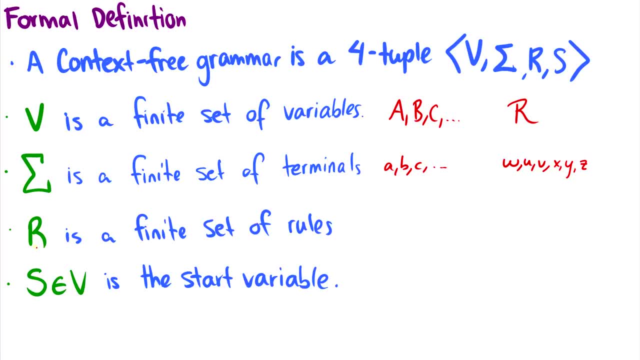 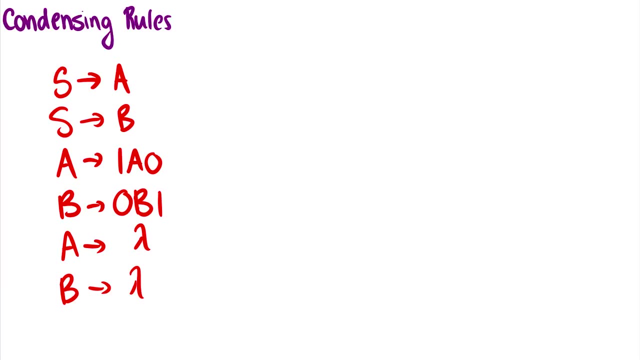 terminals in rules. r is a finite set of rules, So we can't have infinitely many rules And we have a start variable, which, in most cases, I'll just call s. Now, the last thing in this video is I'm going to show you how to condense rules. 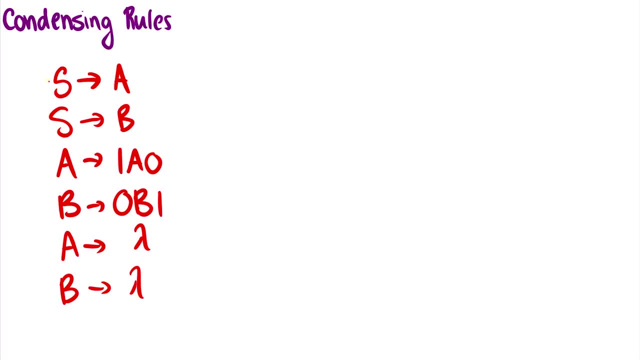 Now it's not very nice if we have s goes to a, s goes to b and these are all separate rules. We want to make them nice and compact. So if we have a in our tree and we want to go somewhere with it, 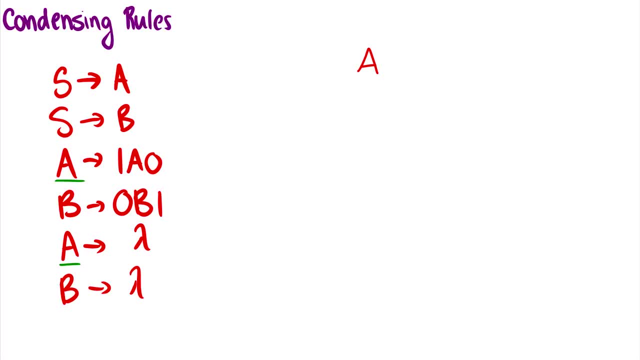 we don't have to hunt down for all the a's and say, oh look, there's one rule number three that can apply and one rule number five that can apply. We want to make them nice and compact. So how do we do that? Well, we just use a disjunction symbol. So I can combine these rules: s goes to a s goes. 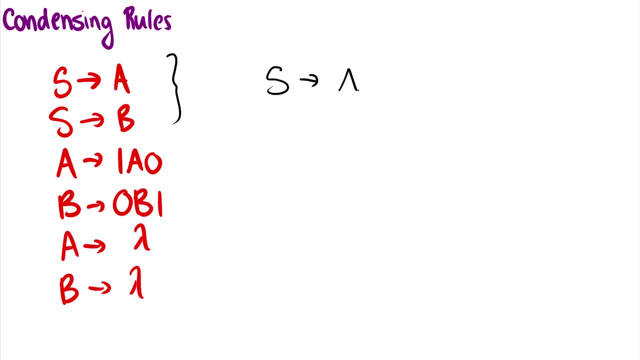 to b by saying that s goes to a disjunct b, with this line in the middle, And this states that either s can go to a or s can go to b. So now for a. well, we have a goes to 1a0 here, The other. 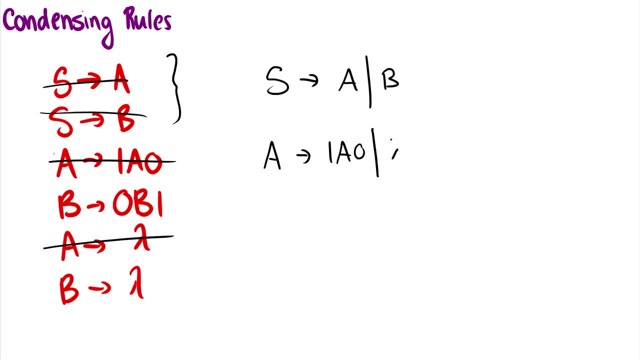 possibility is that a just goes to lambda and terminates. So we can condense it like a goes to 0b1 or it can go to lambda. So that's condensing rules. And that was it for the introduction to context-free grammar. Now there's one thing I want to point out that will be important for the next.